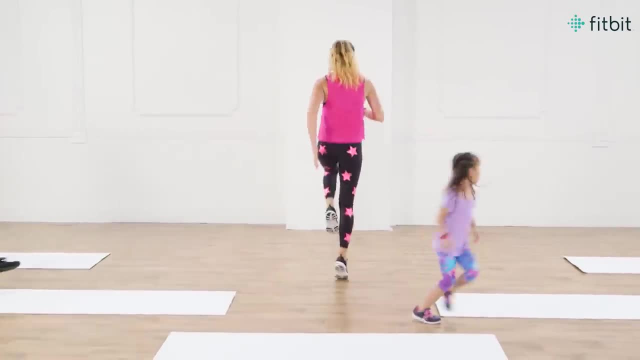 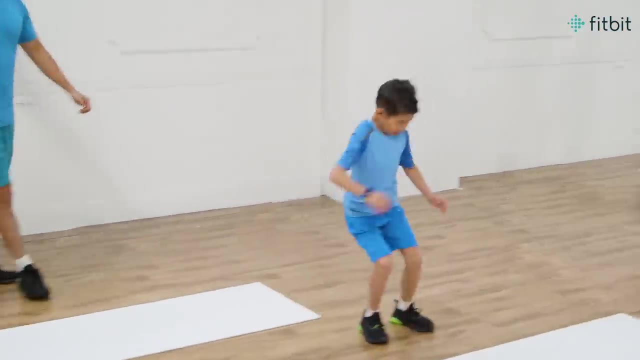 skipping in place. Maybe give each other a high five. There you go right there, bud. Good, Give each other a high five as you go. bye, Good job, Alright, and bring it back to the middle. Hopefully you're feeling warmed up. We're gonna start with our first fun activity. 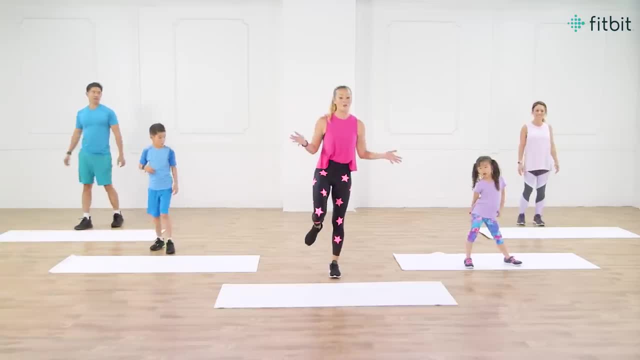 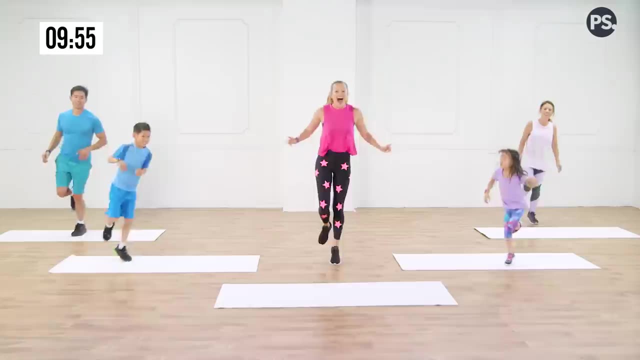 and that's the single-legged hop. Okay, So we're gonna balance on one foot and we're gonna start to hop on that one foot. Ready, Here we go. go good, you guys look awesome. i love the fitbit ace too that these kids are wearing, because it. 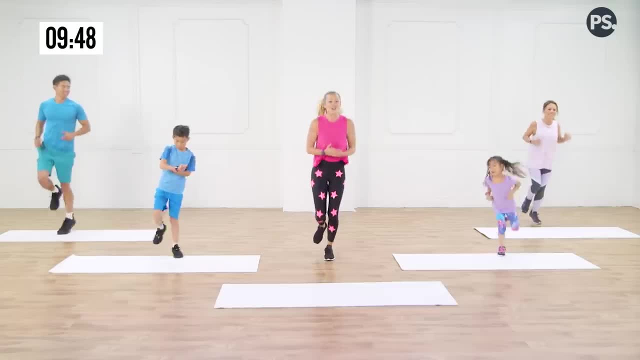 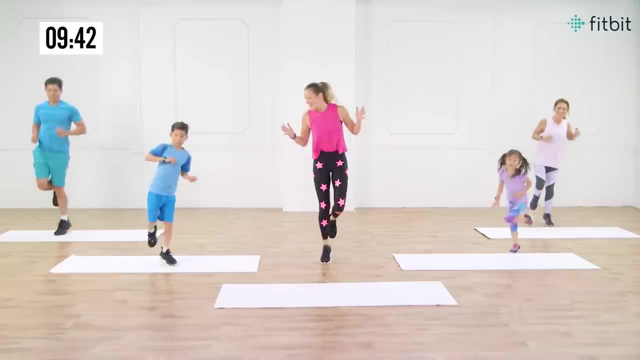 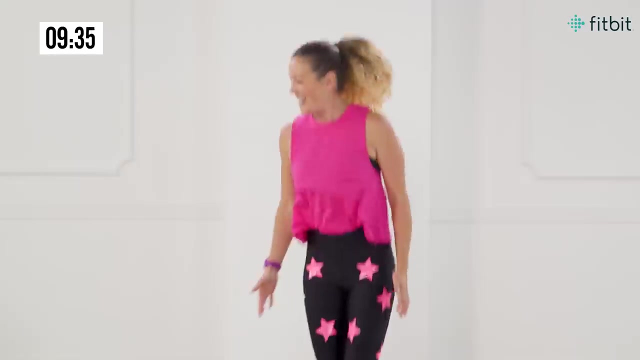 makes activities fun and rewarding. kids can earn virtual badges and trophies and compete in step challenges. right, yeah, good. switch legs to other side. are you guys up for some friendly challenges today? yeah, good and relaxed. so today we're gonna have some friendly competition. we're gonna do some. 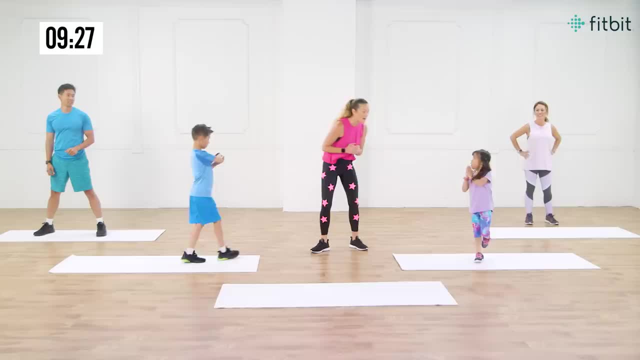 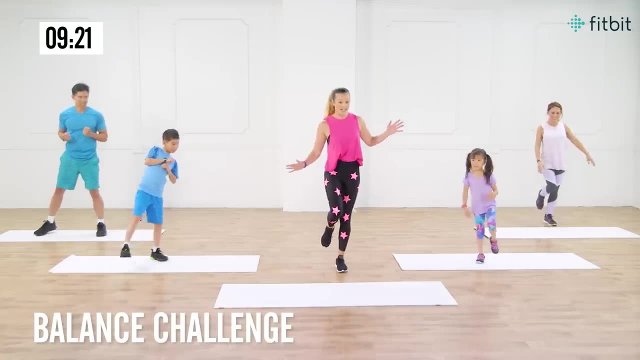 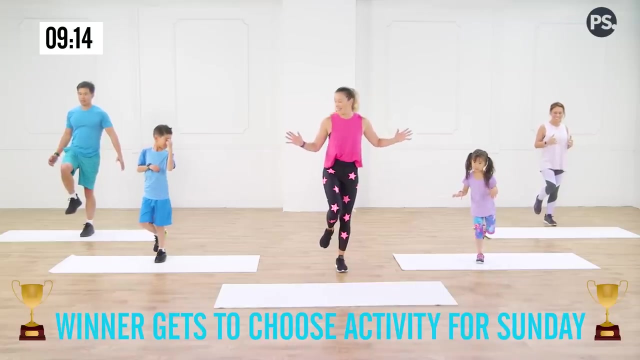 challenges. you're gonna earn a special prize if you're the winner. all right, so our first challenge is gonna be a balance challenge. we're gonna stand on one foot and we're gonna hold that position for 30 seconds. the winner gets to pick the family activity on sunday. good, so hold it there, try not. 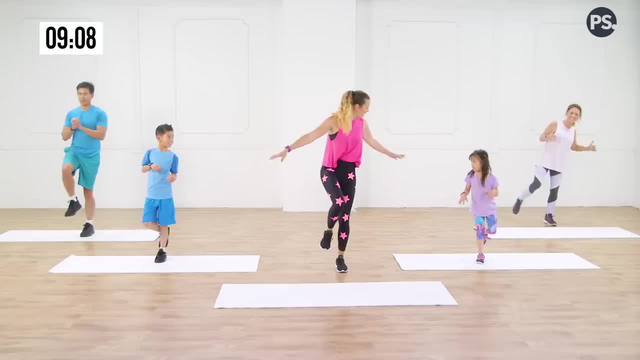 to let your other foot touch up. keep your foot off there. there you go. you can't touch anything with that other foot for the whole 30 seconds. move your hands. you can. you can move your hands. that's actually harder to do. so. if you do hand, maybe she gets extra points because she's moving. 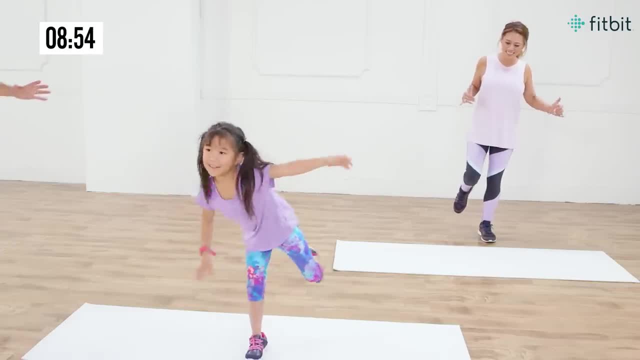 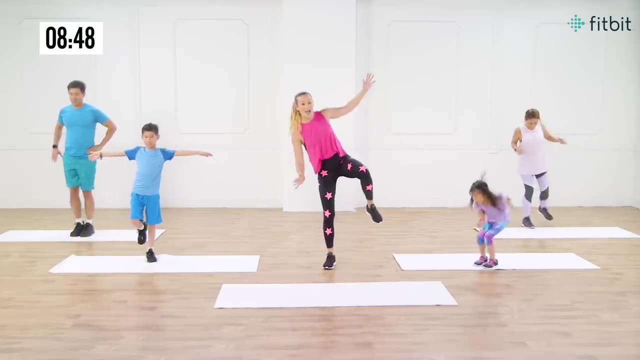 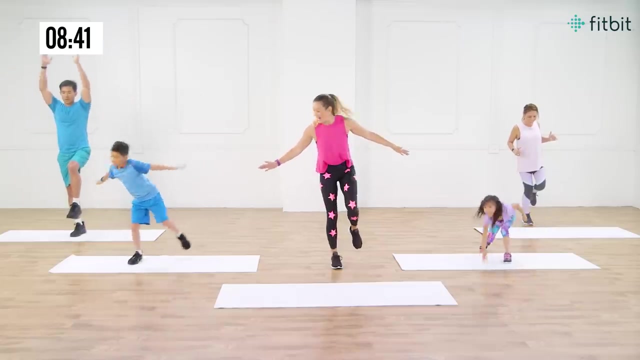 other parts of her body, which makes it much harder. good mercy, that looks great. oh, christian's got it too. extra points and switch legs- other leg- we got to hold it for 30 seconds now. are you guys both balanced equally on each side? looks like it's harder on that side. huh, because sometimes it's. 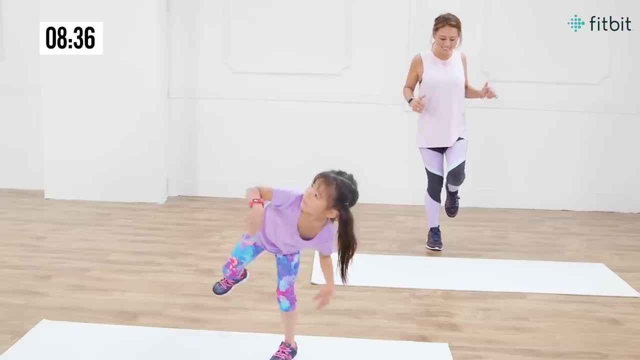 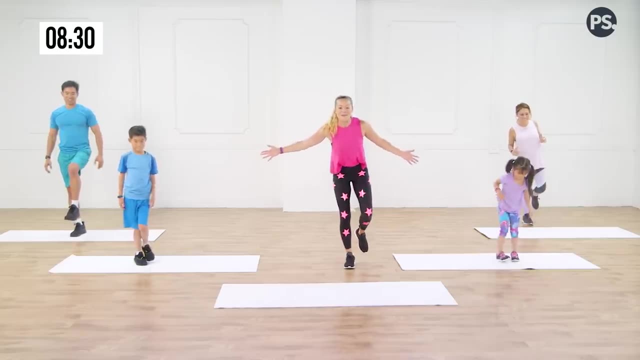 harder on one leg versus the other is that. is that side harder for you? yeah, a little bit. look at this. you guys have perfect balance over here. the whole family is going to win this challenge. how about you guys? are you feeling it? who's winning? good, hold it there a couple more. 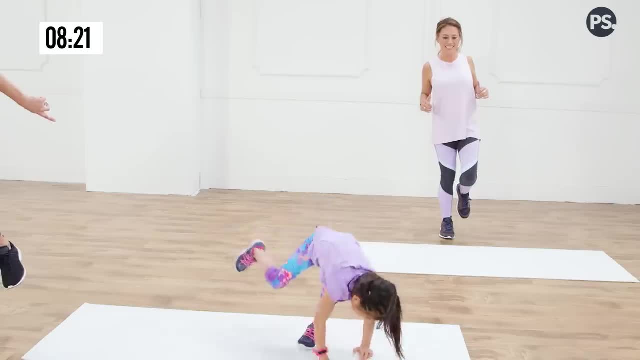 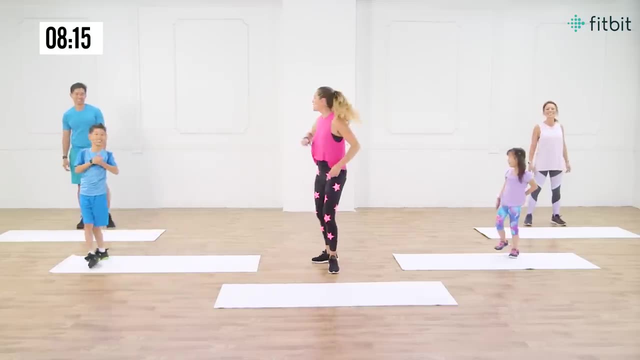 seconds, get that foot off the floor. there you go, and okay, i think, the winner's back here- that all day you guys get to pick the family activity. what's your family, your favorite family activity? running, running, oh that's awesome, good for you. steps, yeah, you can count your steps, that's so. 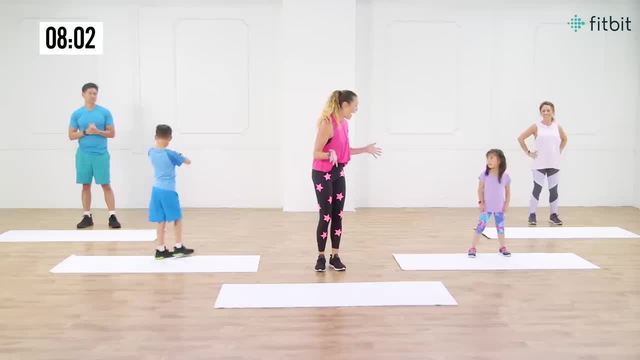 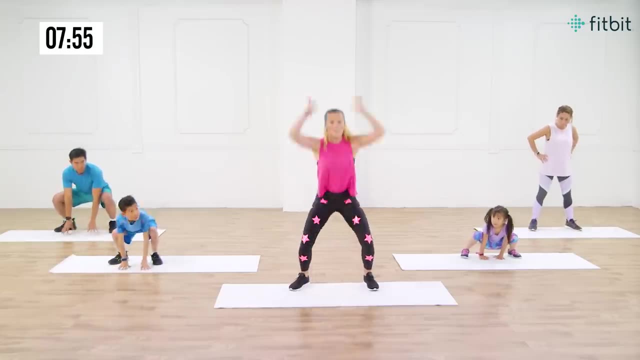 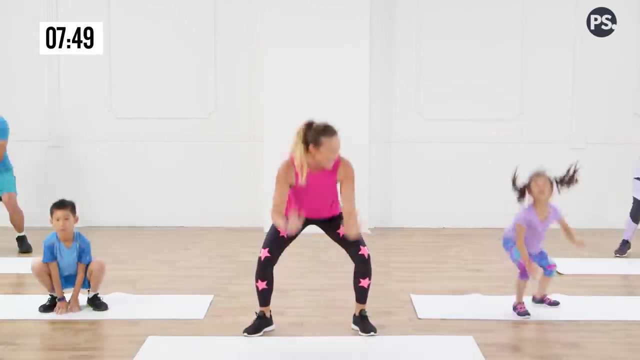 good, all right. now the next one we're going to do is our frog hop. okay, so we're going to come on to the mat because we're going to go down into a squat, touching the floor and then jump up towards the sky. ready, go up and down. so we're going up and down, touch the floor, reach towards the sky. 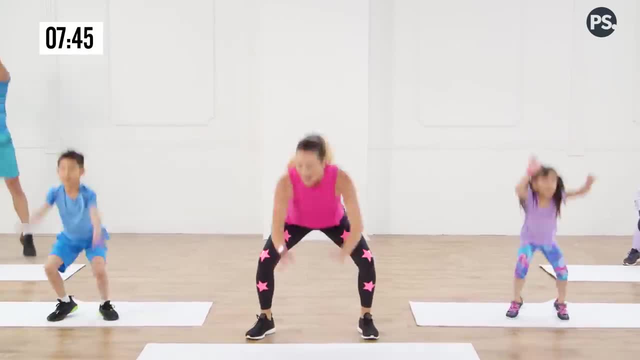 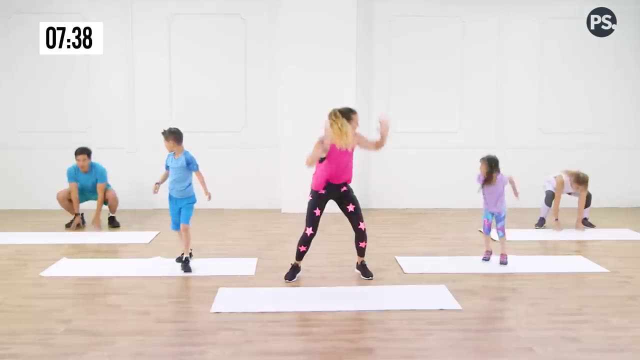 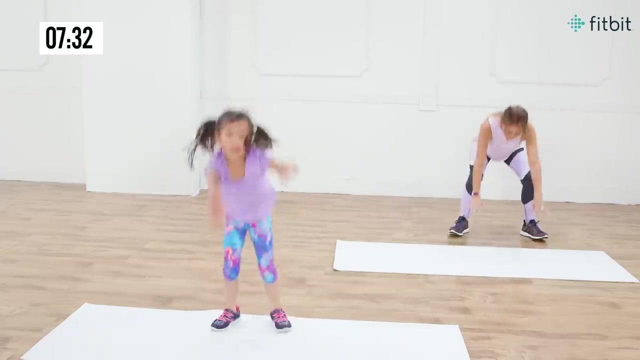 good. look at how high you're getting. remember the frog hop makes you get low and then it gets you off those feet, gets you jumping towards the sky. whoa charles is going crazy. look at you- mercy. good job girl. awesome, keep it going. a couple more seconds here we're working those legs, we're getting strong. good job, keep it going. 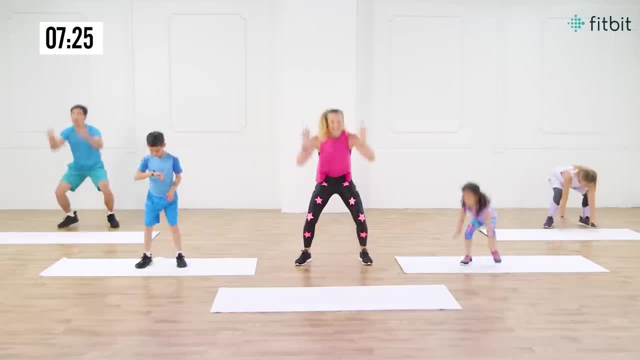 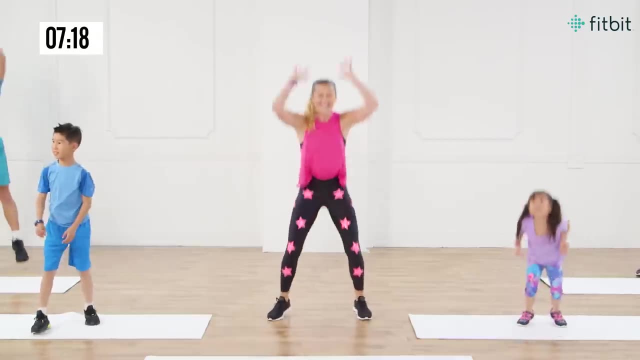 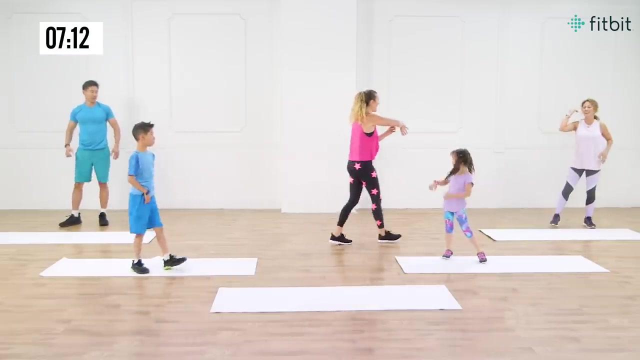 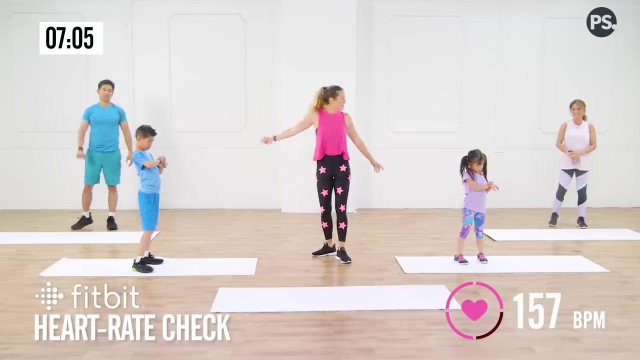 frog, hop it all over, keep it going. almost there, that's it. you've got it. last two, last one. all right, take a moment. take a moment. what do we got for our heart rate? do you have a heart rate over there? my lin, i'm at 122, 113.. 157, 157, that one gets the heart rate spiking. all right. 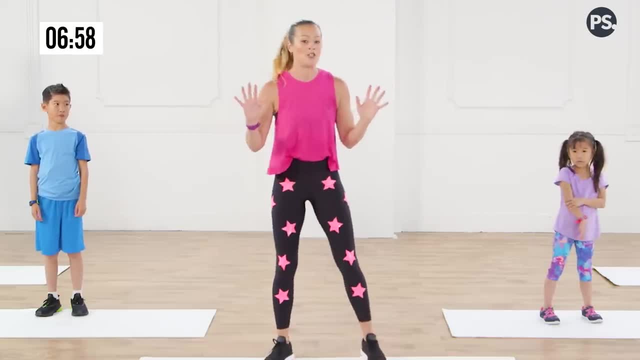 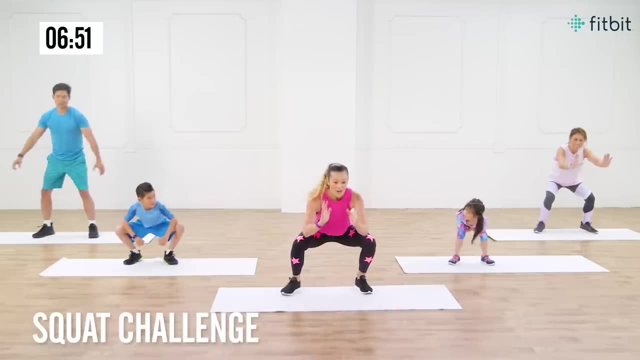 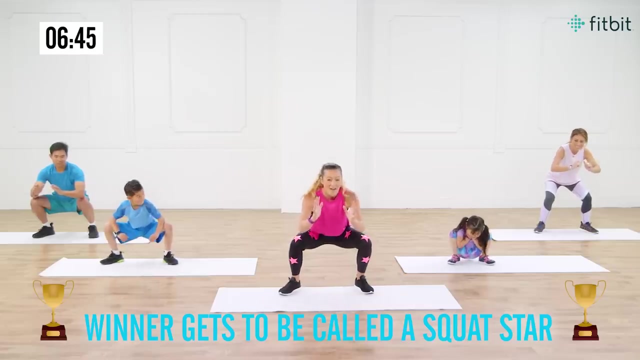 guys. now this next challenge. we're gonna go down into the squat hold, so we're gonna hold it in the squat position like we were doing the frog jump, and the winner of this one is gonna be considered the squat star. so you guys are going to get that label of squat star if you can hold it. 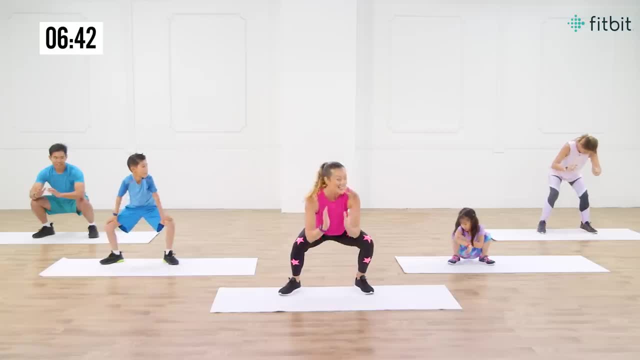 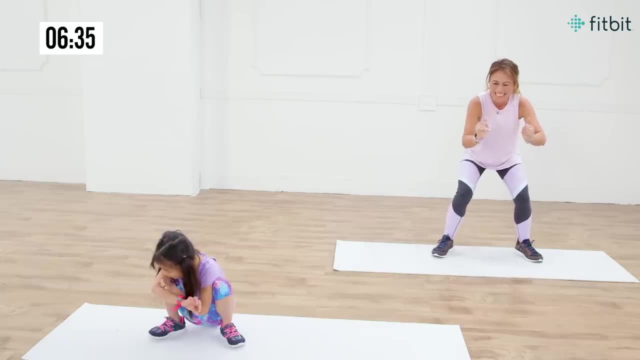 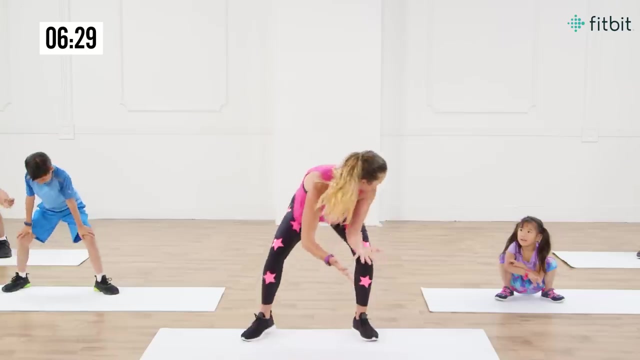 for the whole entire minute. this is not an easy challenge. look at mercy's just hanging out. she doesn't even know she's in a challenge. squatting, right. this is just fun activity. looking at scabs or freckles- whatever you can do, right, what are you? 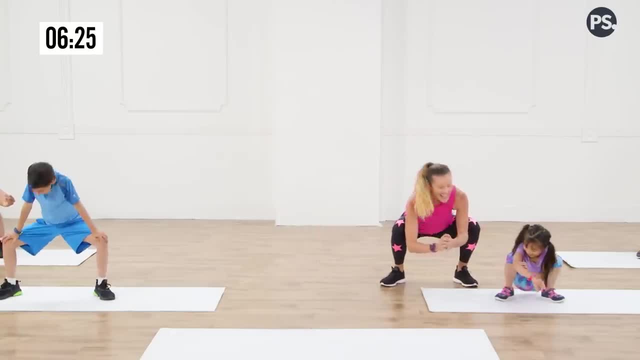 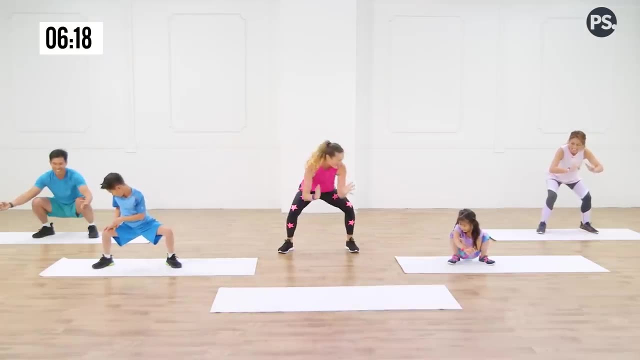 doing over here. huh, are you enjoying this one? yes, are you guys enjoying this one? this one's not easy. get that, get that down. get that down. good, you gotta be considered the squat star. you gotta hold it. that's it. look at, charles, the depth on that squat is no joke. 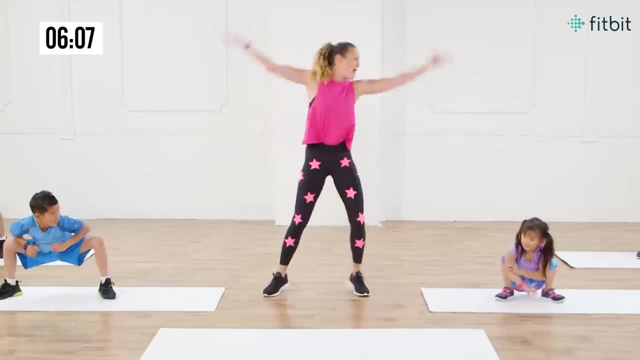 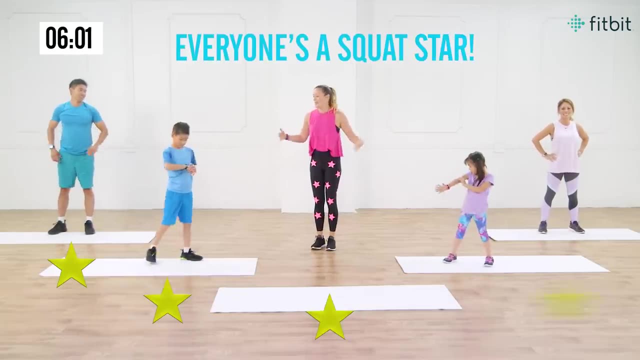 look at you, she's got the perfect deep squat right there and come on up everybody. that was pretty awesome. i would have to say that everybody's a winner on that one, and so everyone gets the squat star title today. okay, badge of honor. all right, now you guys know hopscotch. does everybody know hopscotch? 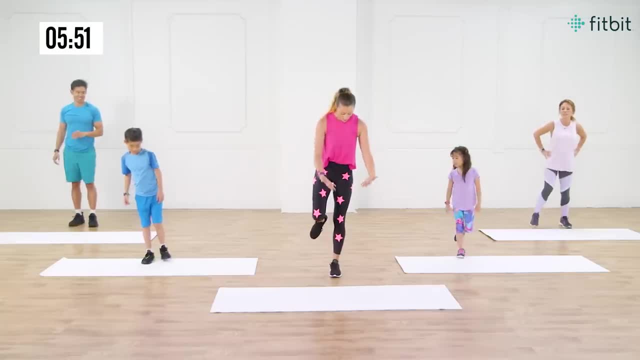 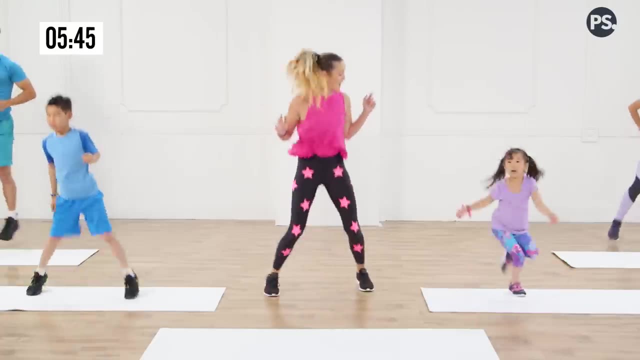 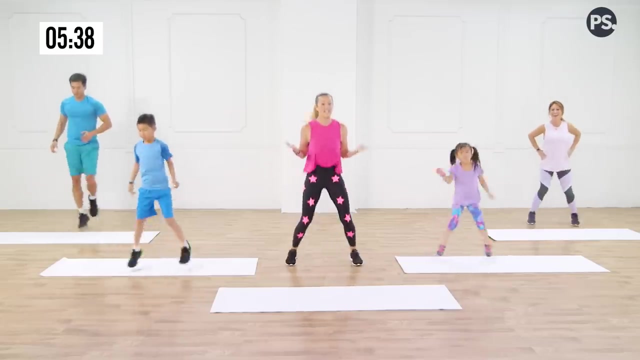 yeah, okay. so hop, scotch. we're gonna try to go one foot to two feet and we're alternating. let's go, we're gonna hopscotch all day long. hopscotch all day, good job, look at that. coordination. now. this is a tough one for coordination, but it's so fun. it gets you playing if you can draw out. 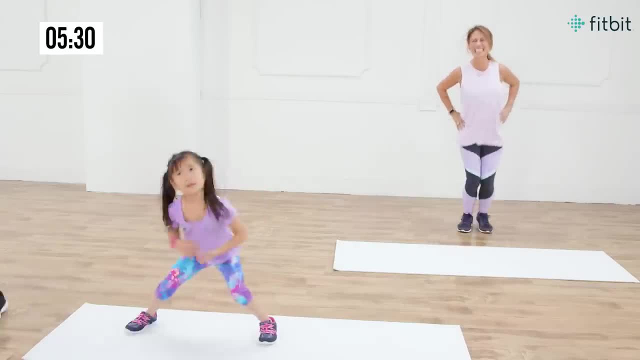 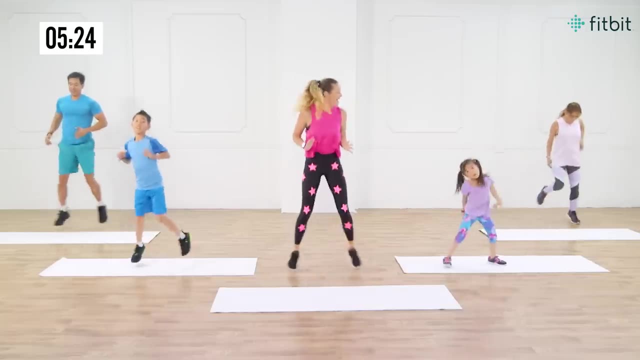 some chalk to make it fun. that's also great. but you can also use your mat or your floor, or just going one to two feet on one foot up on the top of your knees. just doing one foot to two feet, Two feet, three, two and one. 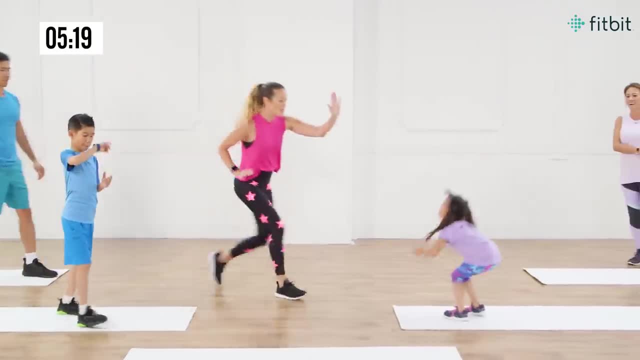 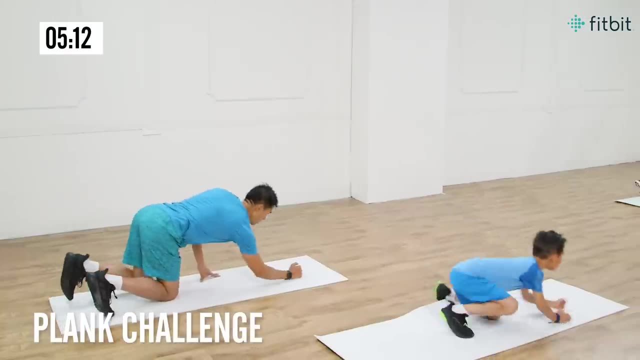 All right, high fives, high fives All around people. good job, You ready for your next challenge. Okay, let's come down onto the floor, and this is the plank challenge. Here we go. let's begin So, without letting your knees touch. 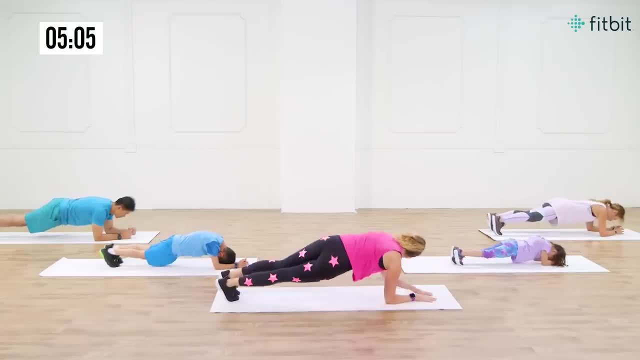 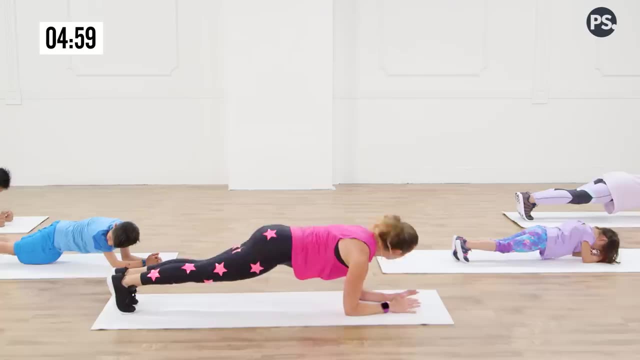 don't let your knees touch. don't let your belly touch. Get your butt up. good, hold it there. You guys look so strong. Now the winner of this one is gonna get to pick what show they wanna watch on TV. 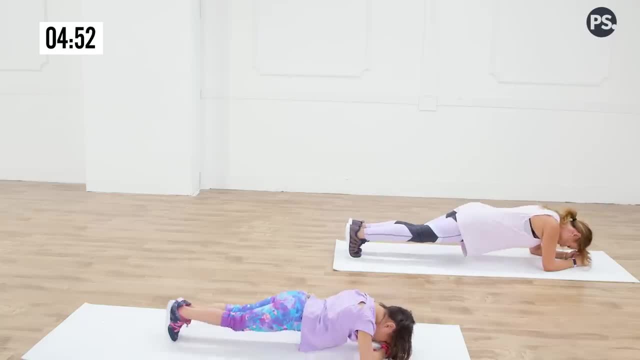 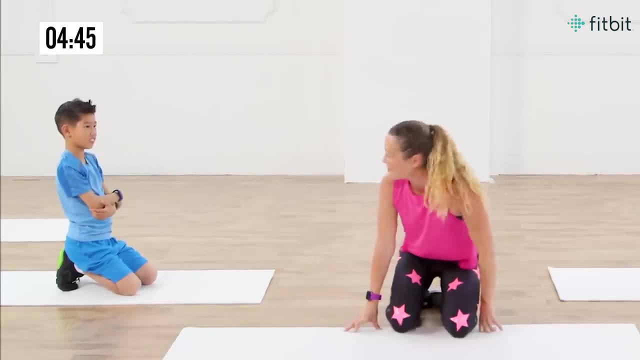 Good job. hold it there. you got it Good and relax everybody. Have you done that before? No, That's the first time I'm so proud of you, because that is a hard move. Mom is dripping sweat. we are feeling good. 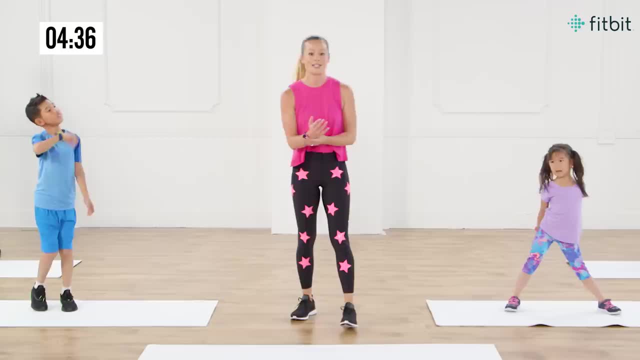 We're gonna come back onto our feet. We're gonna go into some jumping jacks. You guys know jumping jacks, right. Who does the best jumping jacks? Who's the best jumping jacks in the family? Oh, I'll have to be the judge of that. 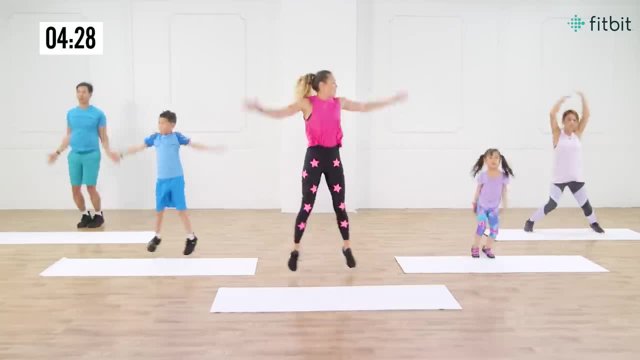 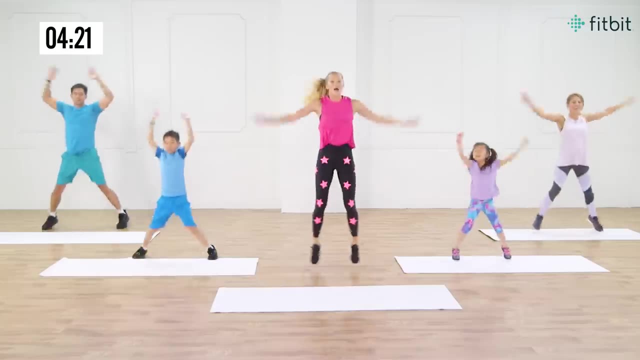 Here we go. let's go jumping jacks, Arms up over the head, jumping off the balls of the feet- Beautiful. Now, this is just a 10-minute workout, right? So it's great to add before or after other activities. 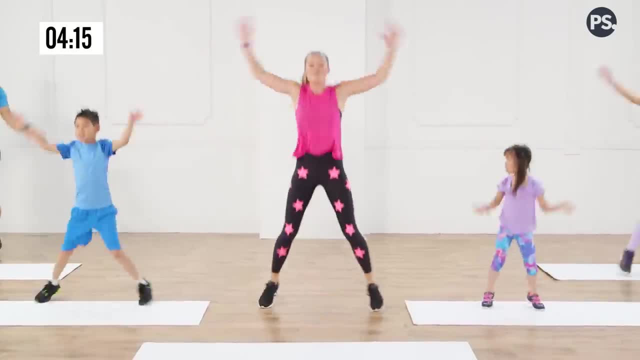 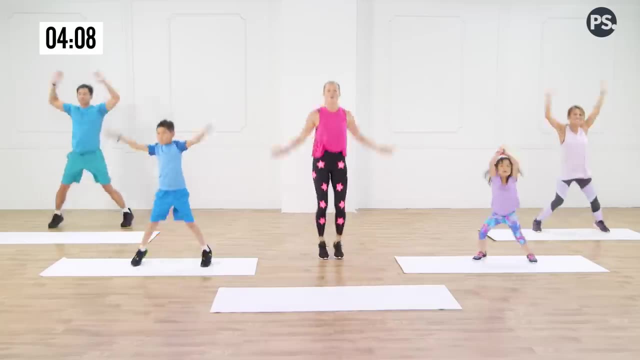 And I love the Fitbit ACE2 that these kids are wearing because it really motivates them to get their recommended 60 minutes of daily activity each day, because they can set a one-hour active minutes goal. I just love that. Come on, guys, you're looking good. 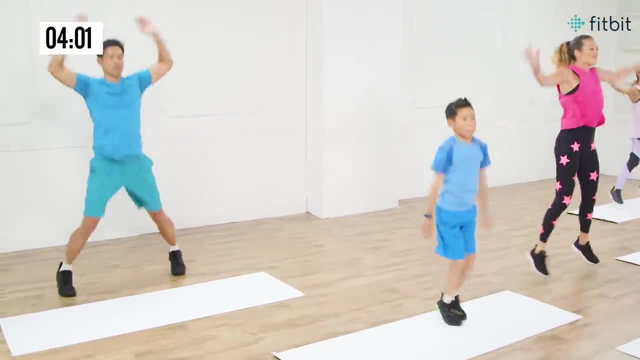 Almost there. Keep breathing. I want to hear that breath And relax. All right, who's up for another challenge? Yes, yes, everybody. Oh, the family. I love the Feng family. These guys are so much fun And they are working so hard. 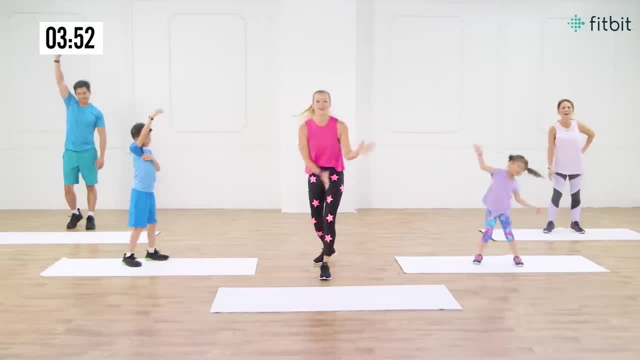 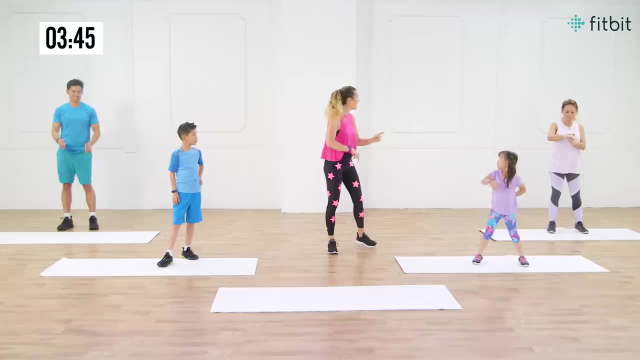 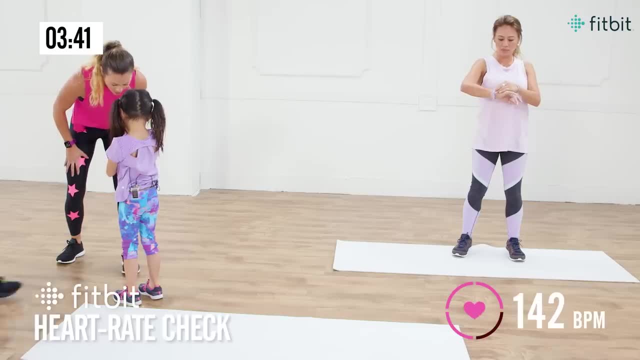 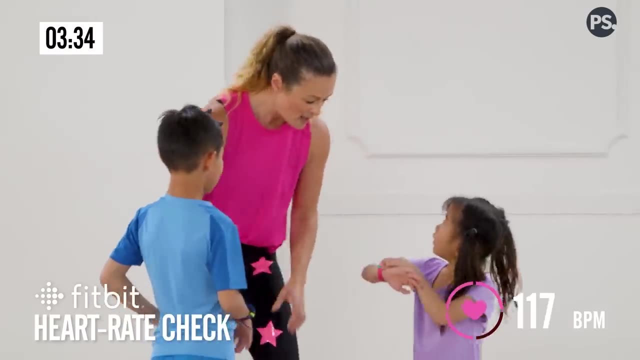 142., 142., 142., 142., 142., 142., 142.. What do I got, Anna? 110.. 110.. I'm at 117.. What do you got? Steps? Oh yeah. 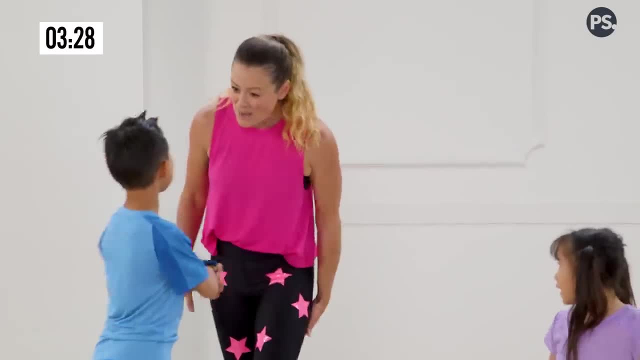 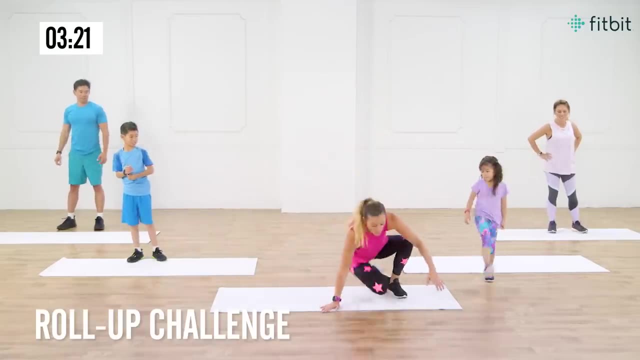 Looking good. 2,800 steps, 3,200 steps- Oh my gosh. All right, here's the challenge for you guys. Now we're going to be on the mats for this one, and it's called the roll-up toe touch. 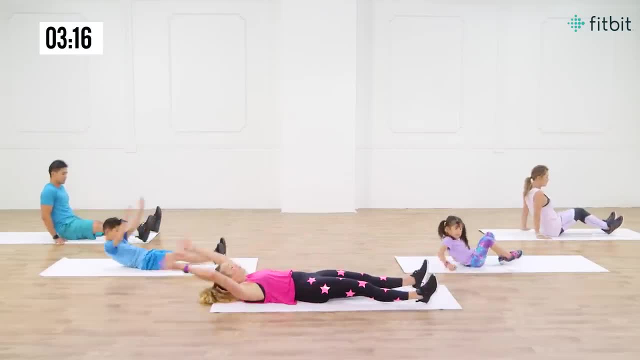 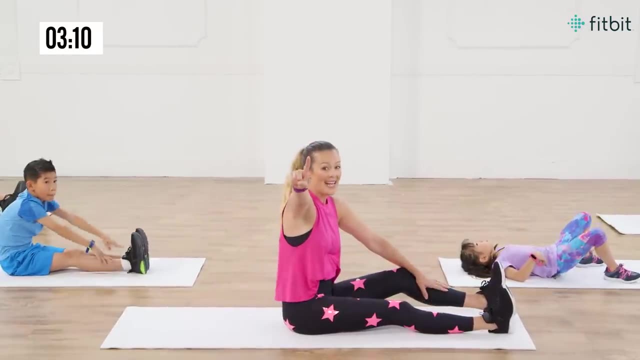 So you're going to be on your back, You're going to roll back and touch the floor and then you're going to roll up to touch the toes And we're going to see how many you can get In one minute. Now, if you can't roll all the way down or up, you're going to do what my Lynn is doing. 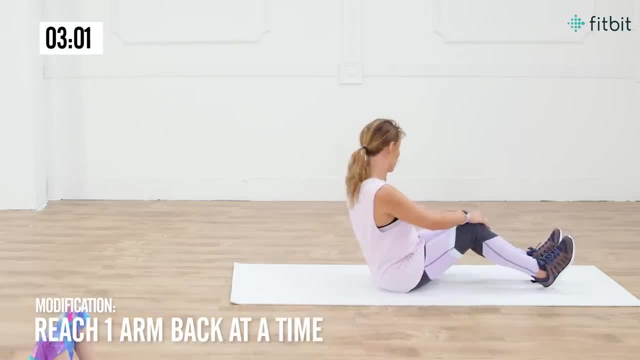 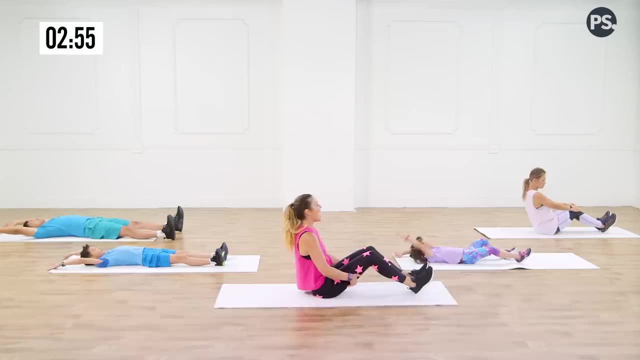 And she's sitting here. She's going to reach back, touch the knees and alternate sides. okay, Going back and forth like that. Okay, everybody on your back And go, Reach up, Touch those toes All the way back. 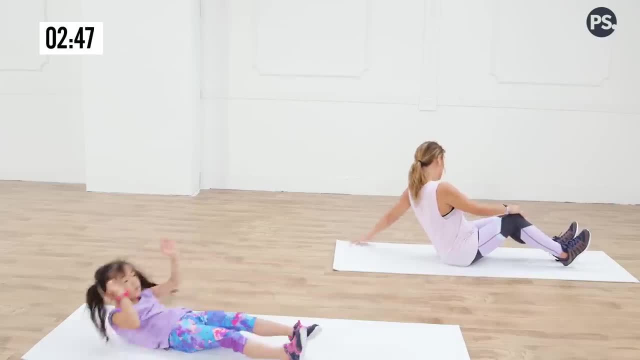 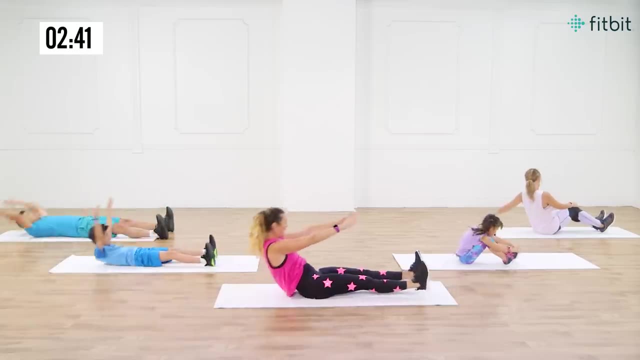 Touch the floor And back up. Good job, you guys. This one is not easy. Keep working hard here. Roll it all the way up. You're working on the core muscles of your body. Is it like sit-ups? Yes, 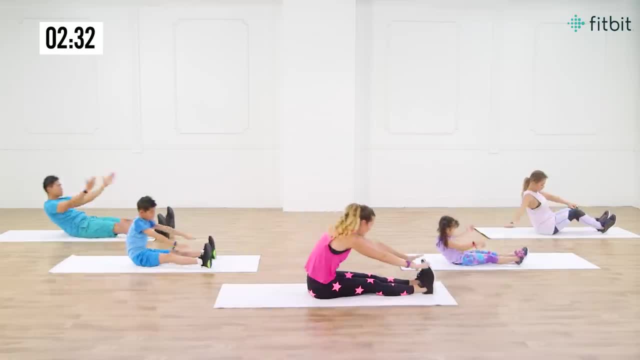 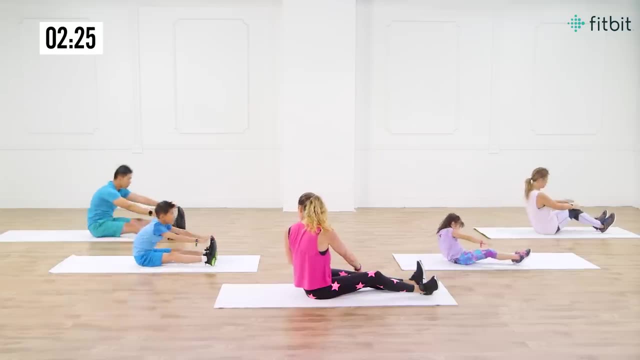 It's a harder than a regular sit-up. You guys are doing the extreme sit-up here And you're getting all the way to your toes. Do you feel that stretch in your legs? Good job, Looking good, Almost there. Are you guys keeping count? 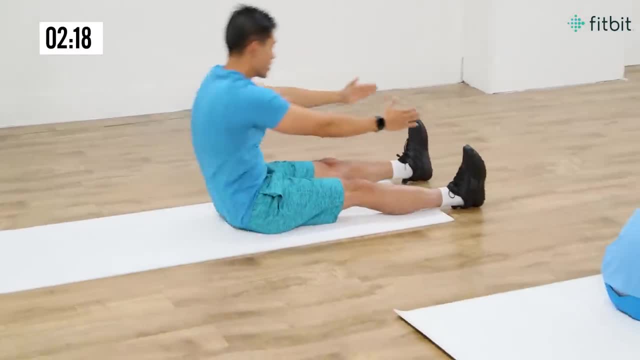 Yep, What number are you on Right now? I'm on Right now. I'm on 15.. 15? Mercy, how many do you have? I don't know. Oh, you lost count, That's okay. 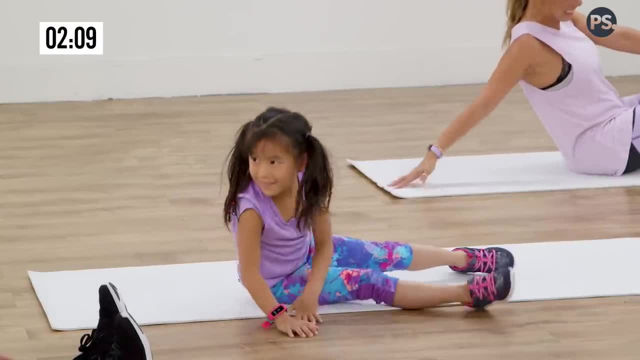 You can count next time we do it. Keep going. Let's see How many you got, Charles 23.. Oh, looks like dad's going to win. Guess what He wins if he gets the most. Guys, you got to hurry up. 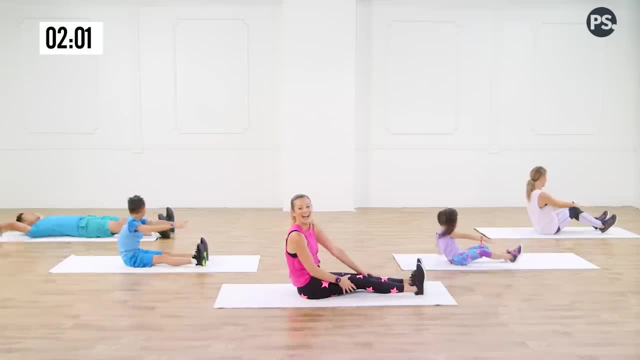 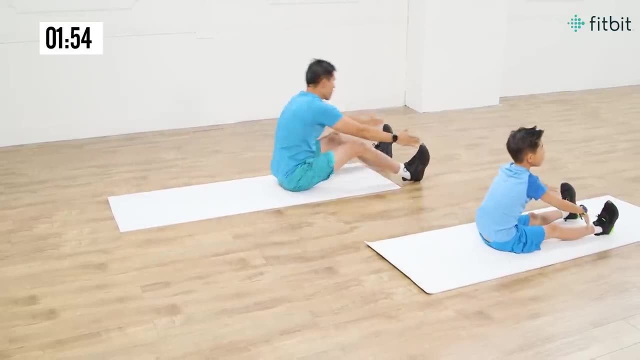 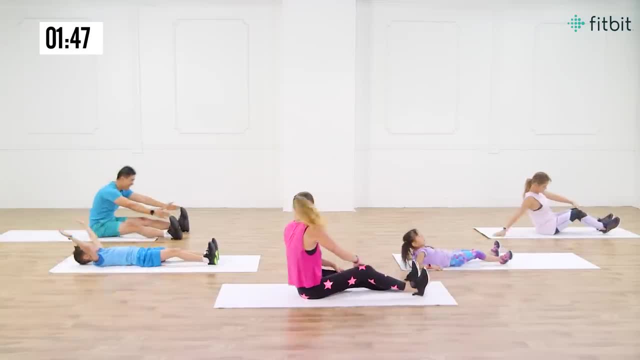 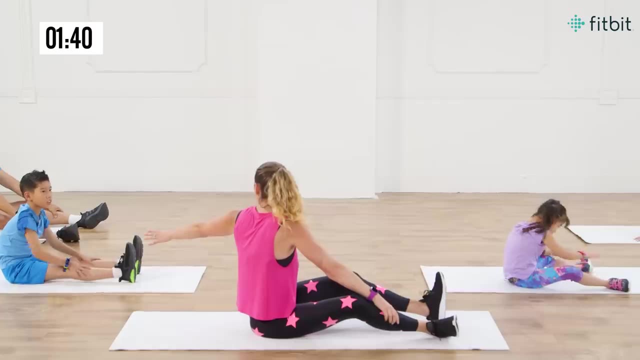 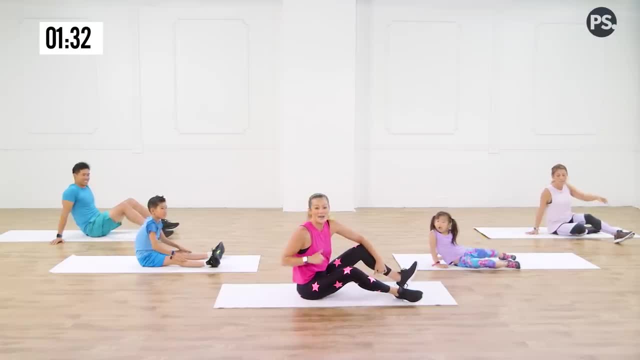 And that's time. It's 20 to 30.. Oh okay, 20 to 30.. So what's your total? Right now, I'm at 35.. 35.. What do you? got Charles 28.. 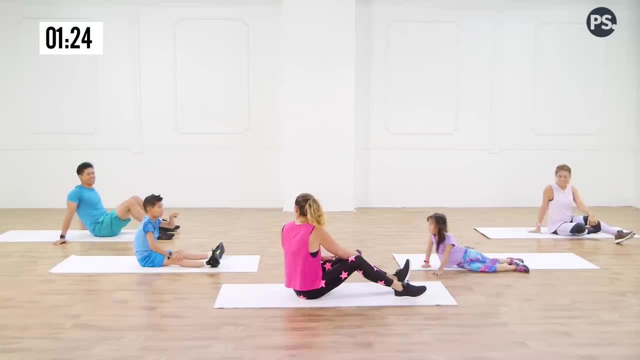 Oh, Oh, I lost count And Mercy lost count. Well, it looks like Christian won. Wow, so you both get to stay up 15 minutes past bedtime. Okay, what a team. All right here, let's come back up onto our feet. 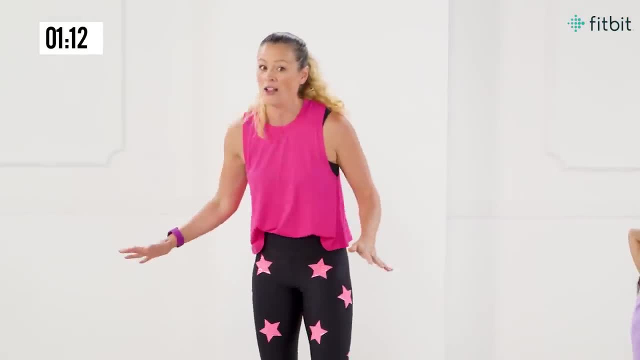 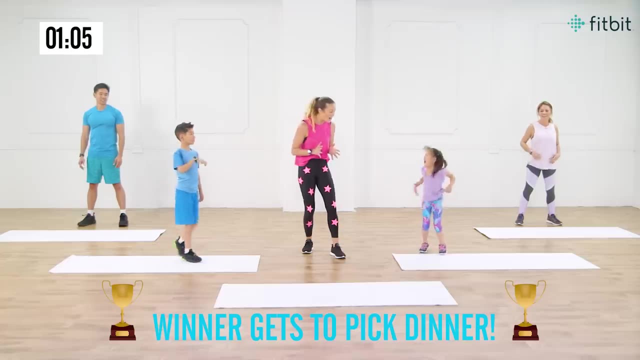 We're going to do our last challenge and that's the sprawl. And the winner who gets the most sprawls in one minute gets to pick what's for dinner tonight. So you guys, you want to do all your best to win this one. 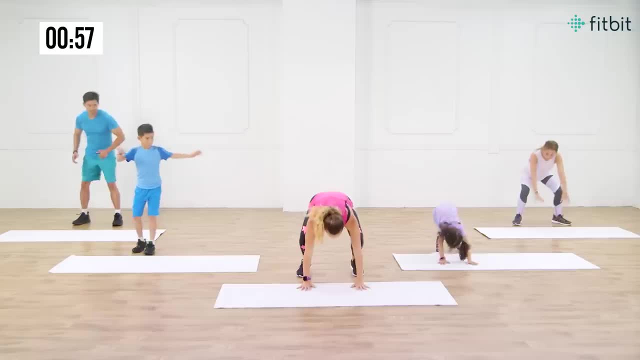 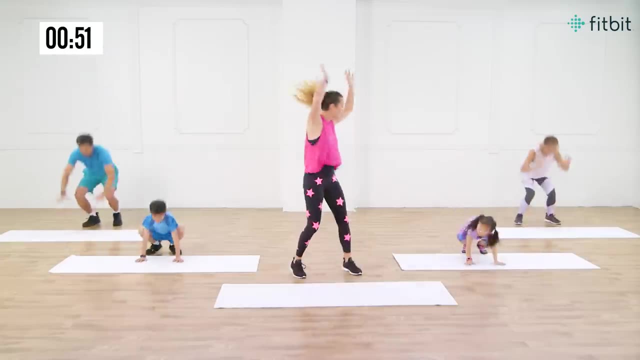 You ready? We're going to come to the floor. We're going to jump out, jump in and jump up. Let's go Get it going. You got one minute. Make sure you're counting. Are you counting? There you go.